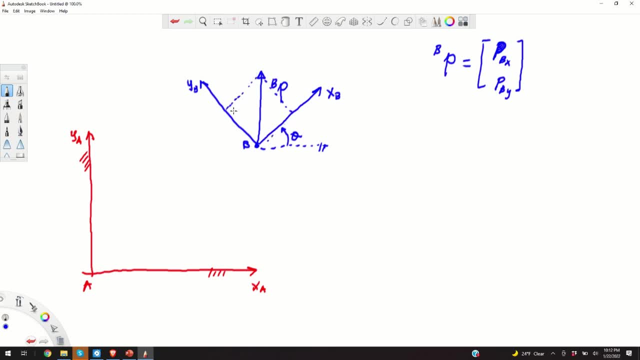 xb projection of the vector Pb. and this is the yb projection of this vector. Now let us assume that the vector that's being sketched like this defines the location of B coordinate system B with respect to coordinate system A. So our goal is to find Pb. 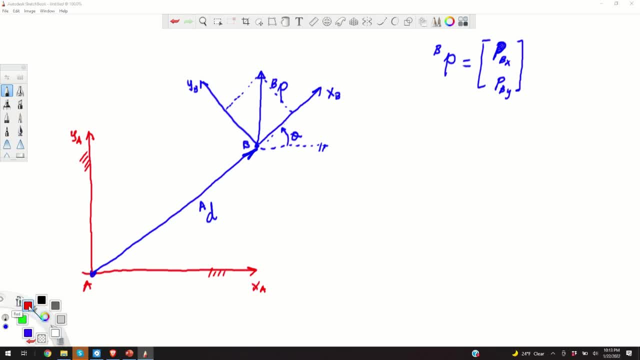 The representation of the vector Pb in the coordinate system A. That is, our goal is to find the coordinates of this vector. So, given angle of rotation, theta distance vector dA, this is basically translation, this is rotation. That is, given rotation and given translation dA and given the coordinates of the vector. 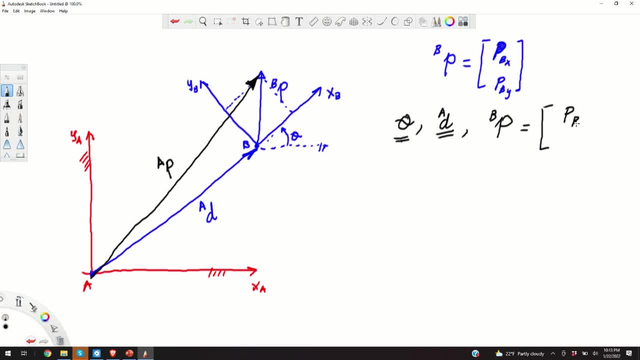 P expressed in the coordinate system B, Pbx, Pby. our goal is to compute or to find the coordinates of the vector P represented in the coordinate system A that are given like this: Sorry, this is basically x and this is Pay. 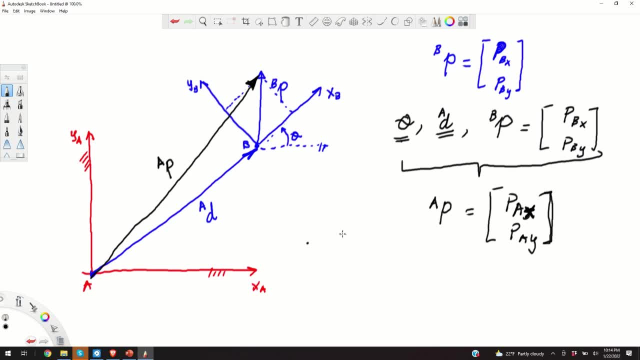 So we will see that it's possible to define one matrix that will take Pb and here one, a newly constructed vector. Its first two rows are Pb And the second, or actually the last row, is 1.. And this matrix will transform this vector into Pa and 1.. 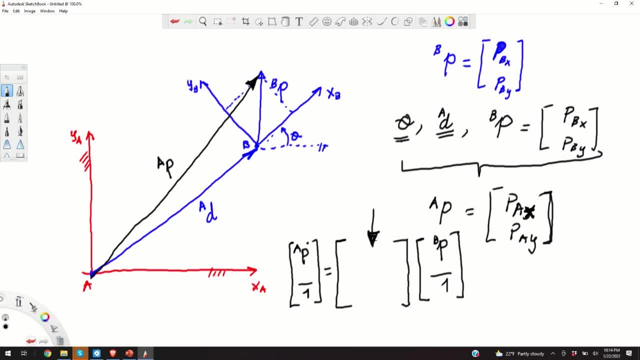 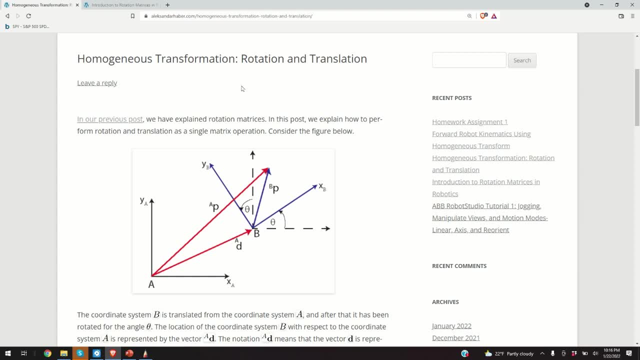 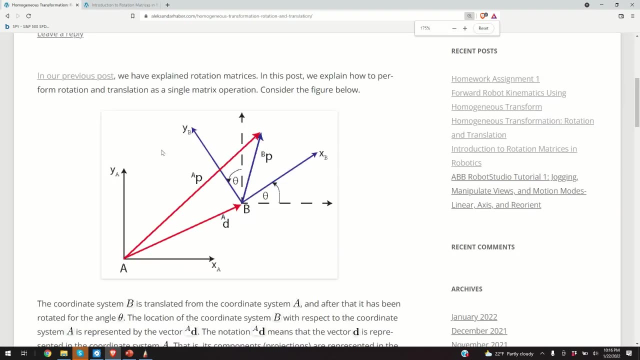 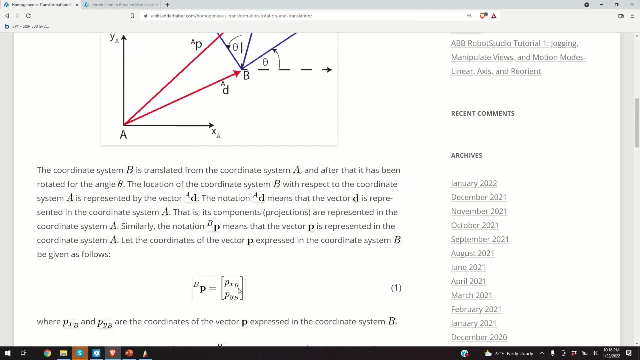 So this matrix is called homogeneous transform. Okay, so let us go back to original post. Here is the picture that I tried to sketch. Now. It's nicely drawn, And please note that I have just permuted the coordinates, or actually the notation. 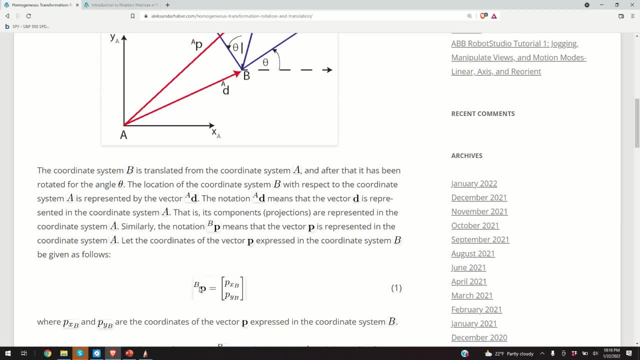 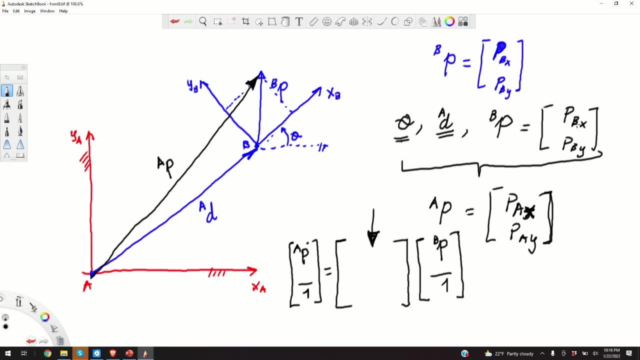 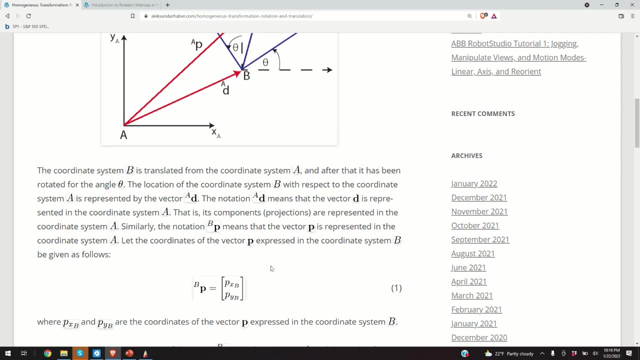 for the coordinates of P represented in B. I just wrote in my previous sketch. basically I denoted this as Pbx. however, in the post I denoted this as Pxb. However, this is just notational difference, So follow the notation written in this post. 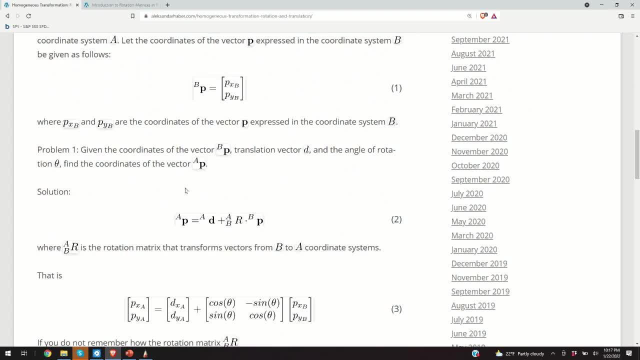 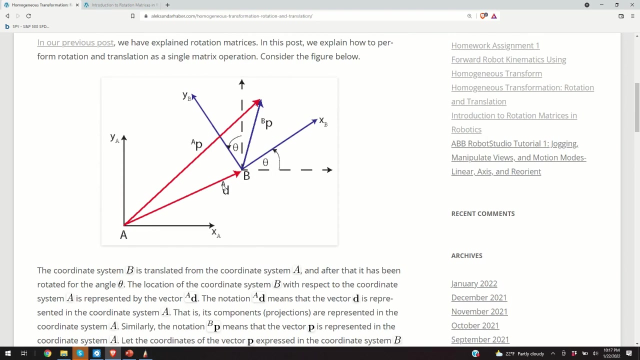 Now this whole transformation, by using the simple vector calculus and simple geometry, can be represented as follows. So the representation of the vector P in the coordinate system A is this vector, which is equal to dA. Okay, That is the representation of the vector d in the coordinate system A plus what? 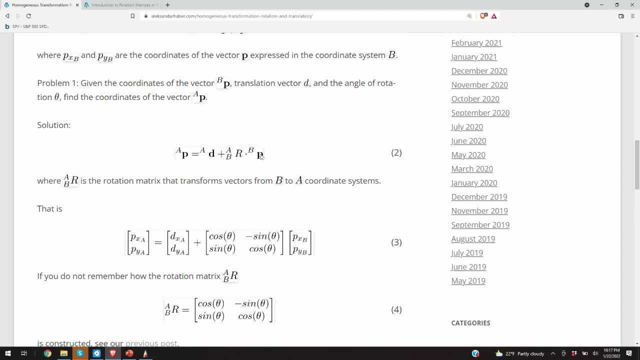 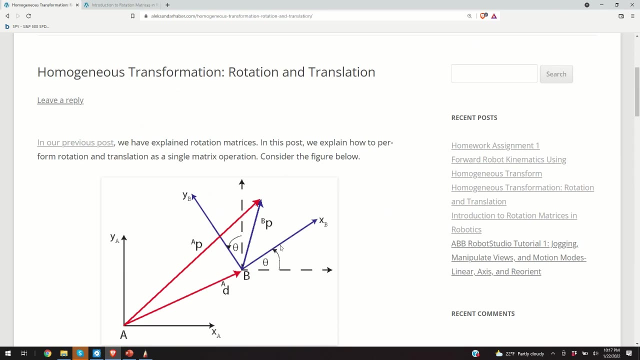 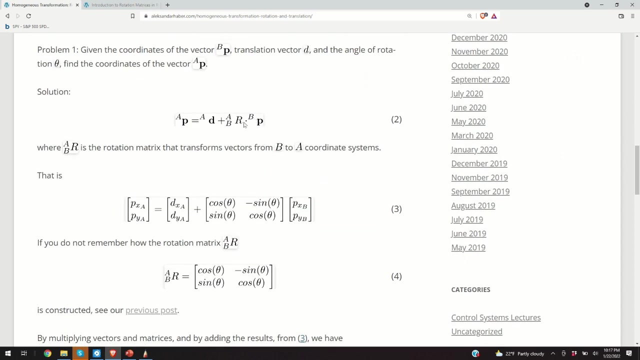 Plus this term. and this term is the representation of the vector Pb in the coordinate system that is sketched here by a dashed line. That is, we basically multiply P, represented in B, by the rotational matrix That transforms B to A. That is, this is not exactly A, However, this is basically. 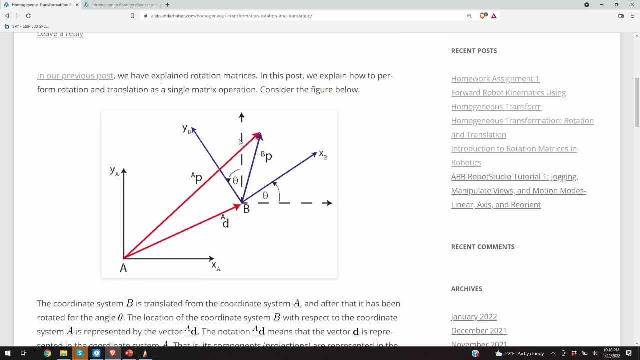 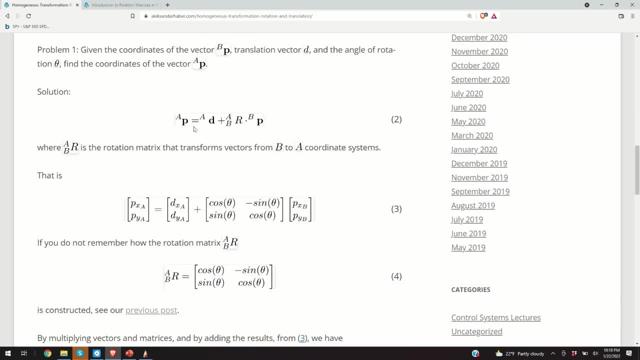 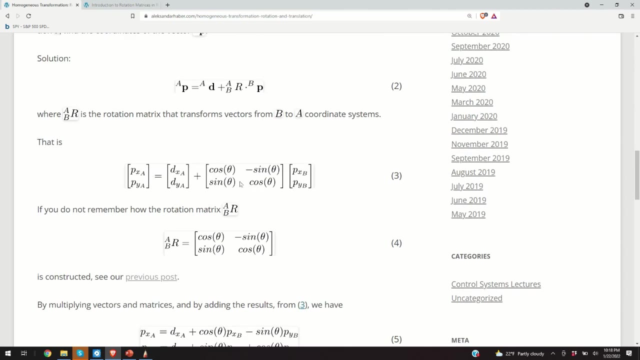 a coordinate system whose axes are parallel to the coordinate system A. So this is how we compute this transformation. That takes into account translation plus the rotation. So if we expand this expression And if we use the definition of the vector Pb, Okay, 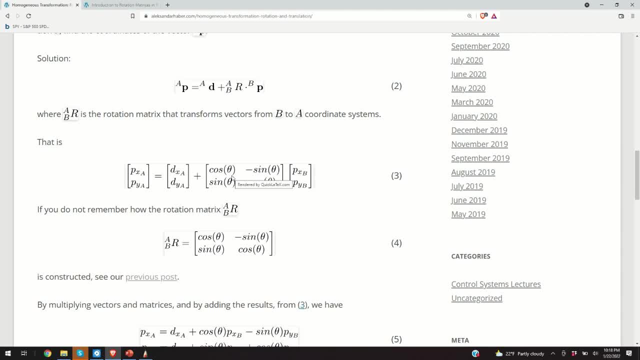 And if we use the definition of the rotational matrix. if you are not sure how this thing is derived, please watch our previous video on rotational matrices. Its link is given in the description below And here. you can simply click over here and the explanation will pop up. 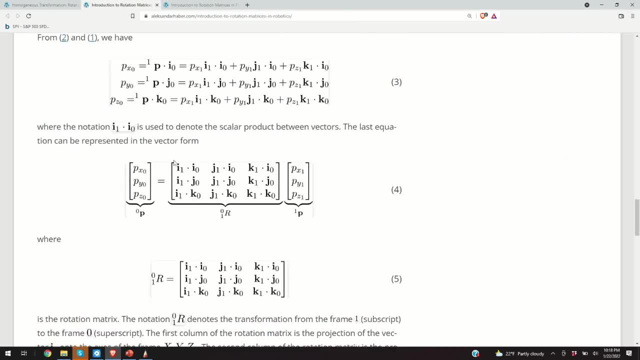 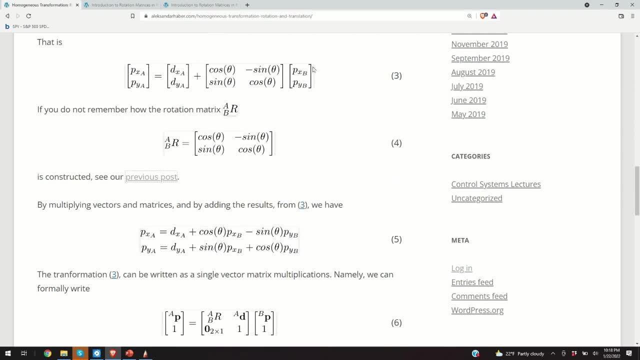 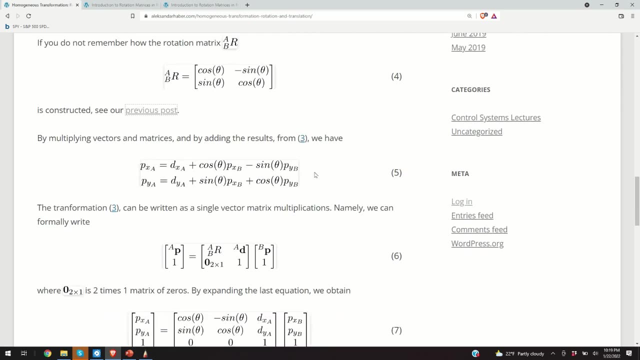 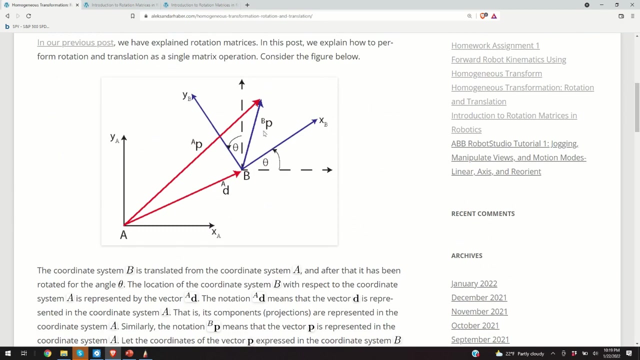 So here is the explanation. and here is our rotational matrix. Here explain how it's being derived. Okay Now, if you plug in these coordinate values and the representations of the rotational matrix, you will obtain this expression. And this expression can actually be obtained without even using rotational matrices, by